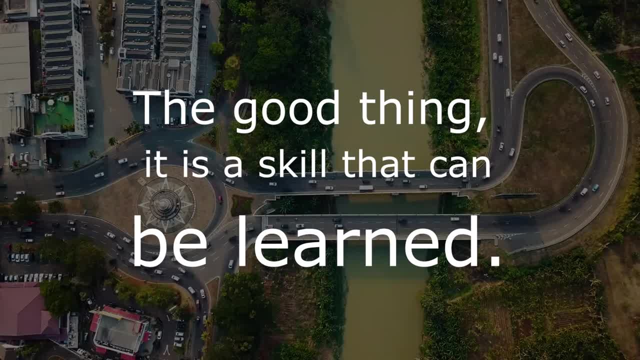 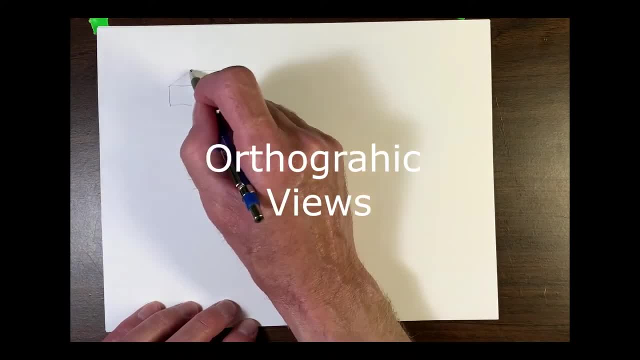 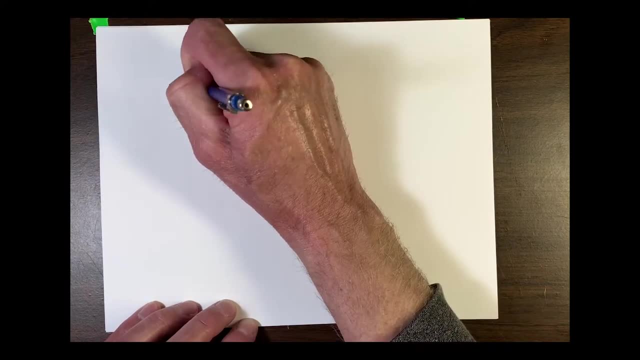 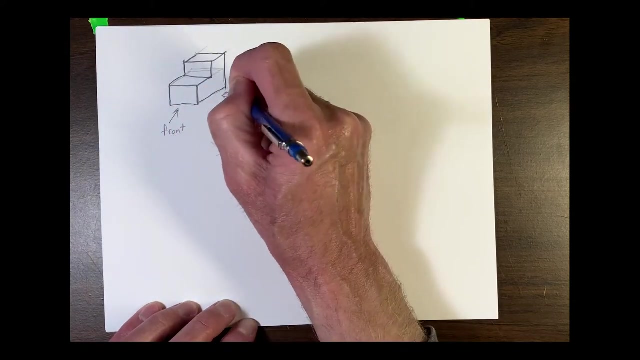 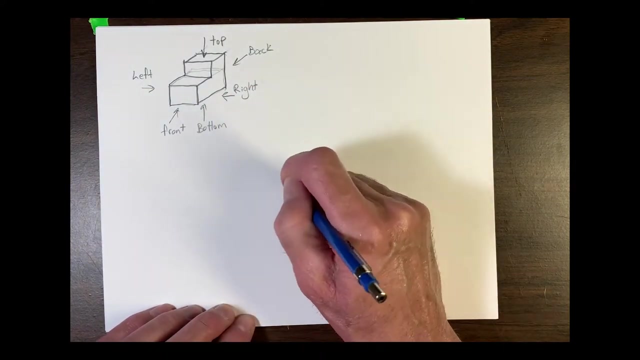 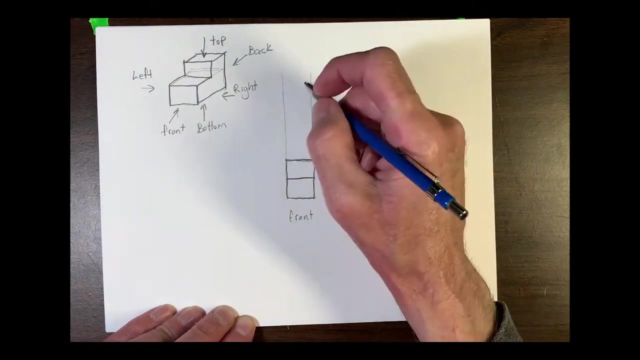 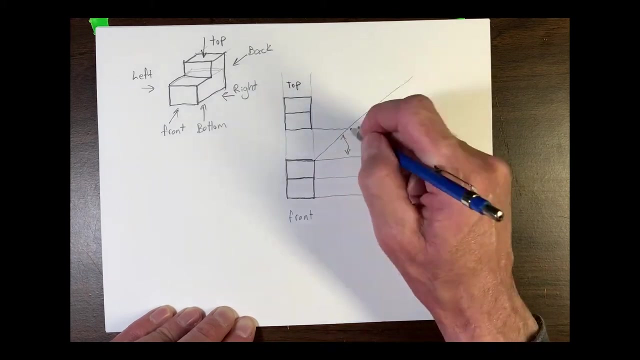 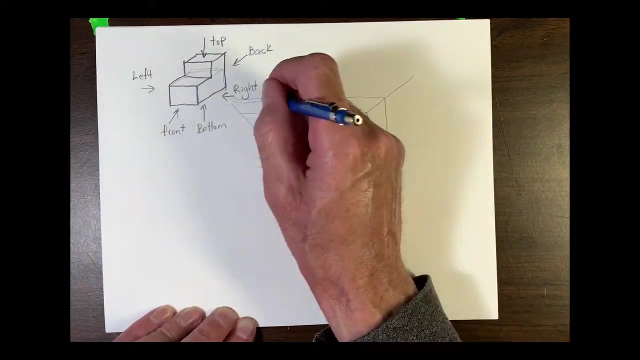 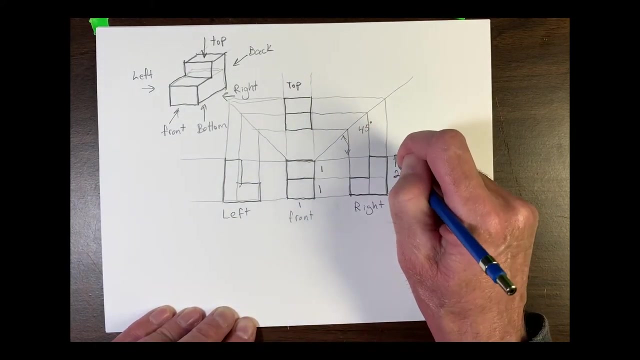 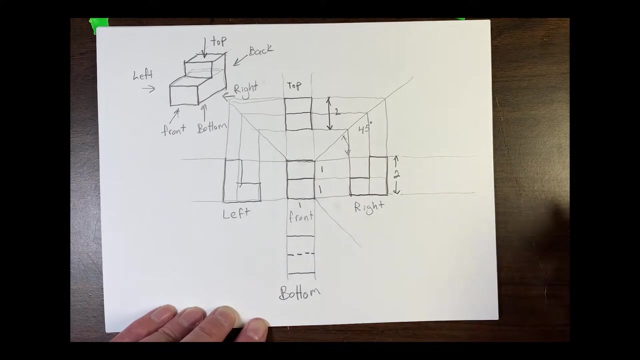 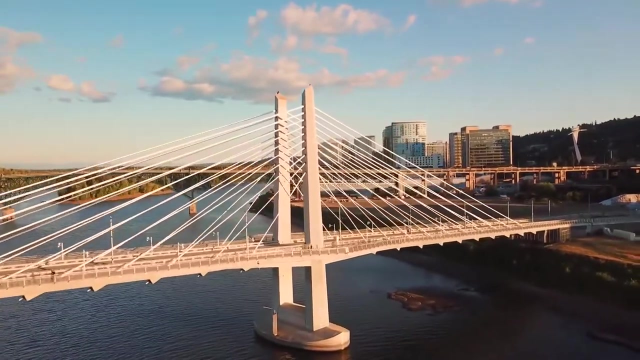 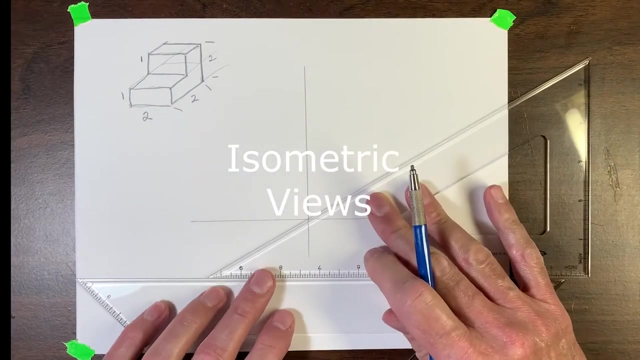 orthographic drawings, isometric drawings and 3d unwrapping. I'm going to show you how to do that in just a few minutes, Thank you, Thank you. Engineers have used isometric drawings for years to show 3D objects on 2D pieces of paper. 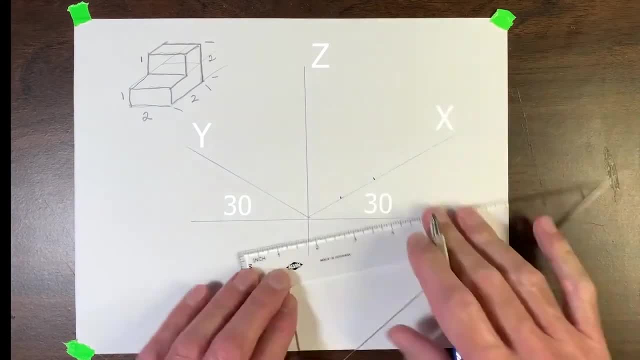 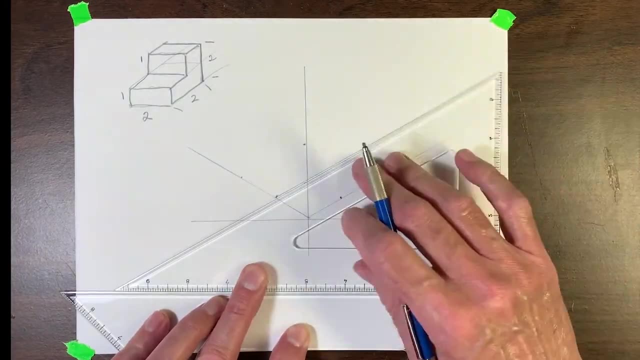 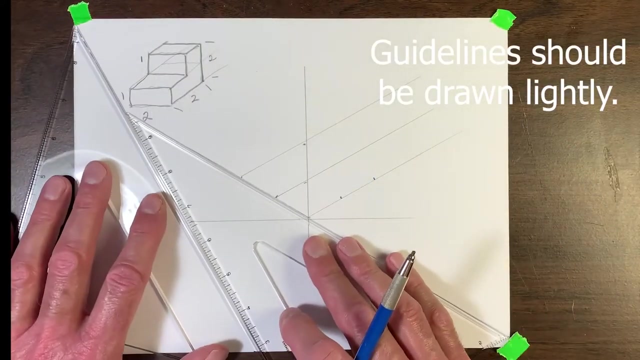 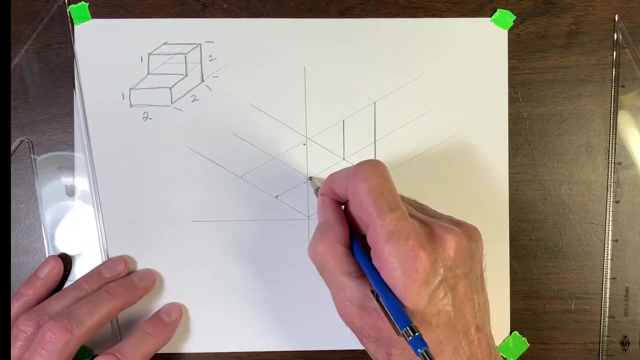 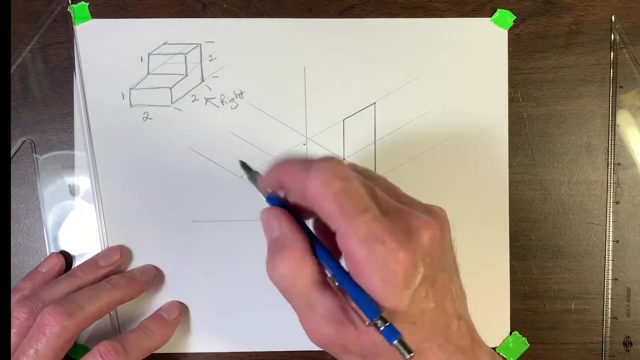 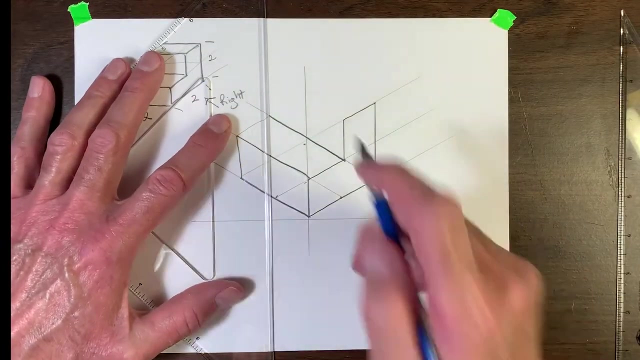 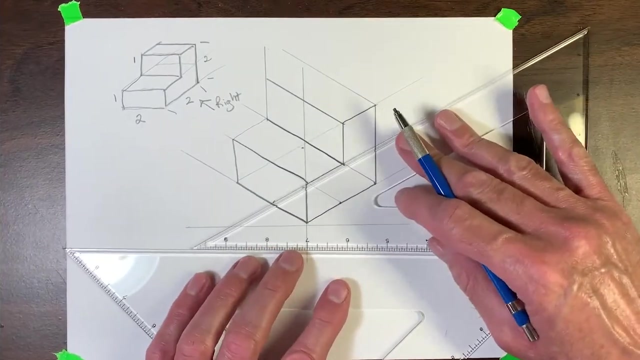 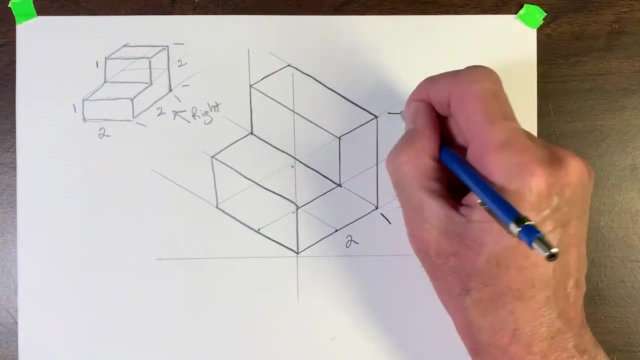 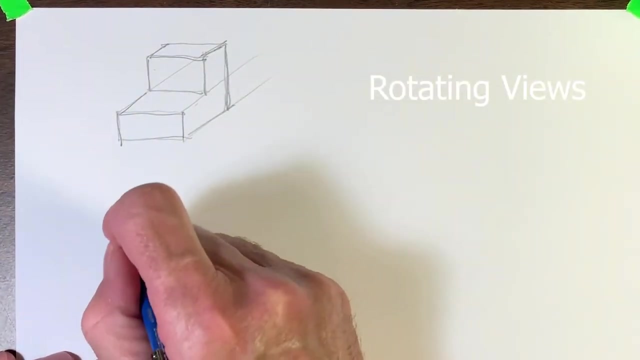 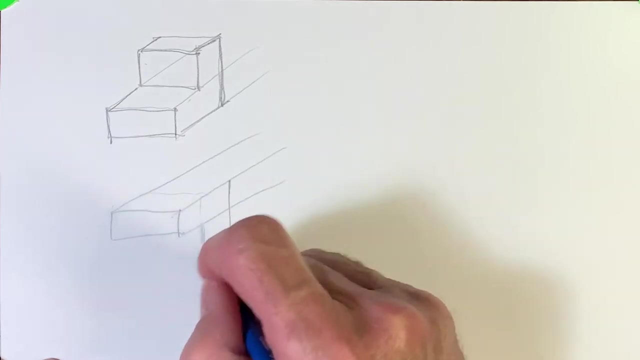 It also allows contractors to build 3D objects out of flat parts. Engineers have used isometric drawings for years to show 3D objects on 2D pieces of paper. It also allows contractors to build 3D objects out of flat parts.